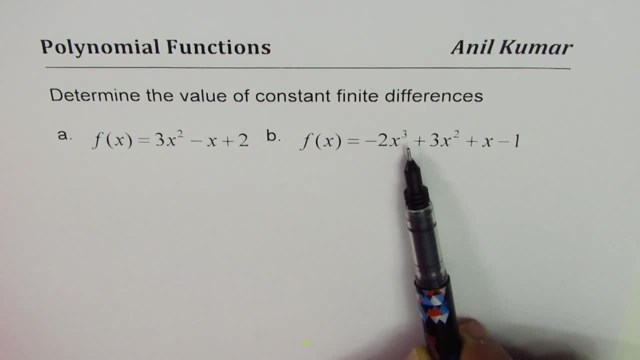 degree 3, then the third finite difference will be constant, correct? So we expect second finite difference to be constant here and third in part B, which is polynomial of degree 3,. right Now, what is the value of this constant finite difference? 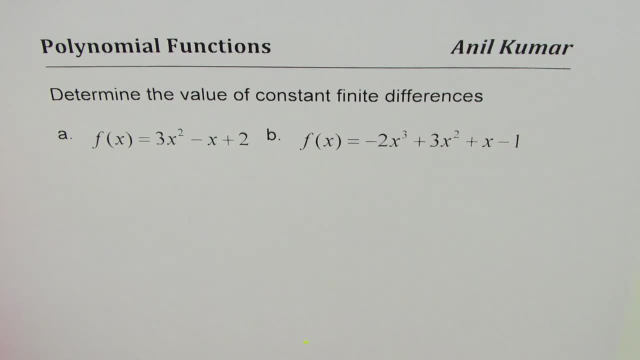 We have a formula which makes it very simple to calculate the result. The alternate method is you can make table of values substituting different values of x, for example 0,, 1,, 2,, 3,, 4, and then make difference table and get your answer. So you can do that to verify the result. 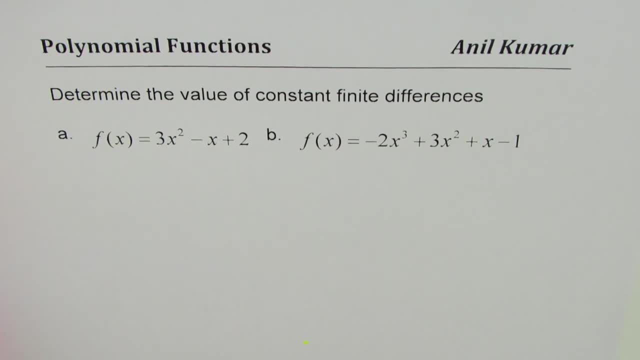 which we are going to show you in this particular video. I'll share with you a formula: Constant finite difference. let me write down the formula here: Constant finite difference. Constant finite difference. greater divide by 2 times x is going to be x is the product of degree. 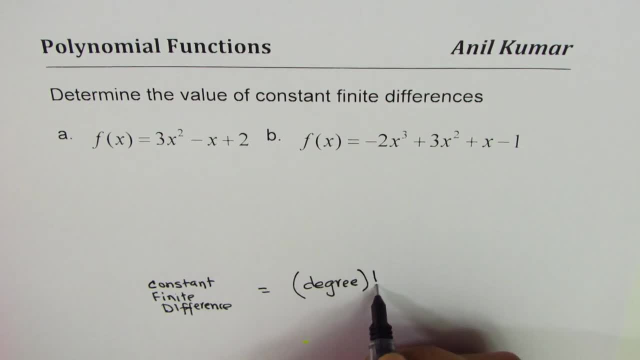 factorial times: leading coefficient. Okay, Now what does this factorial means? Let me explain that also. Factorial really means if I have n factorial it means it's product of n times n minus 1 times n minus 2, so on till. we can write 2 and 1, till 1, where n is a whole number. right. 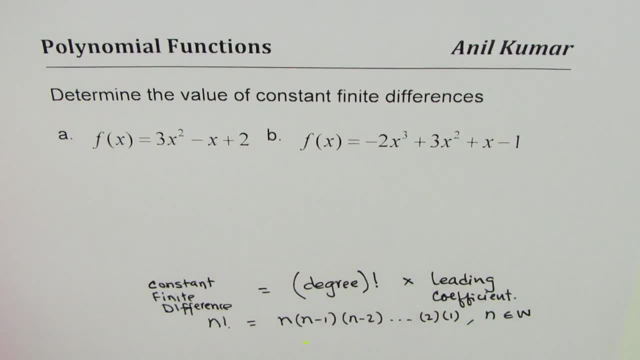 So n belongs to whole numbers. So that's the meaning of factorial. Now you know the formula, I'd like you to pause the video, answer the question and then check with my solution To verify. you can also make table of values and find which constant, find what constant difference value is. okay. 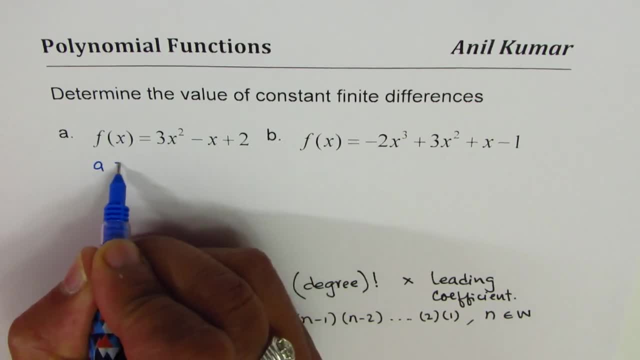 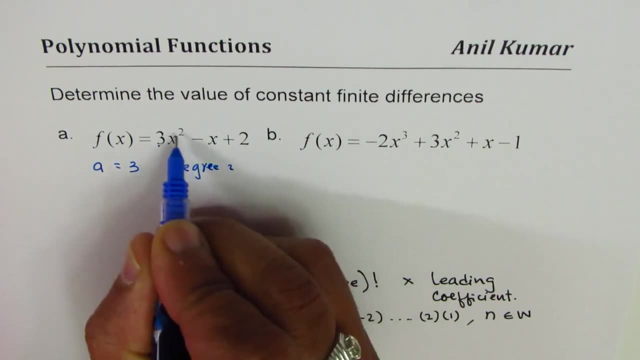 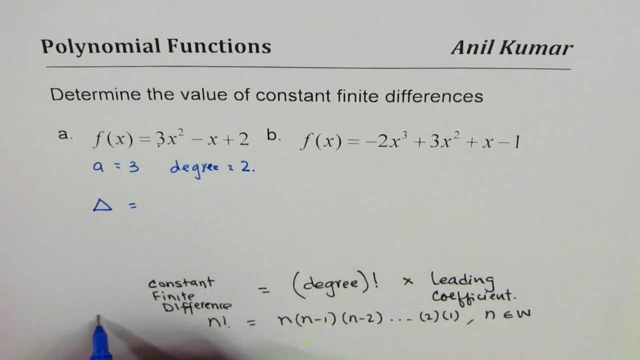 So, for the first one, what is the value of a? The leading coefficient is 3. for us, right, Leading coefficient is 3.. And degrees, Degrees: 2, right, And therefore the constant difference. let me say, this constant difference is equal to: 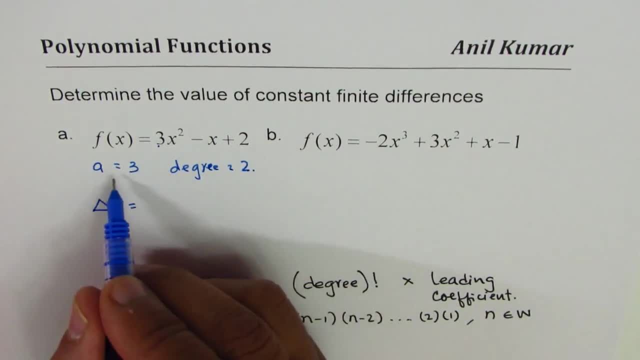 2 factorial times 3, or you could write a times that either way. So we'll write 3 times 2 factorial Degree of 2, right 2 factorial. So that really means 3 times 2. factorial means 2 times 1, right 2 times 1, is it okay? 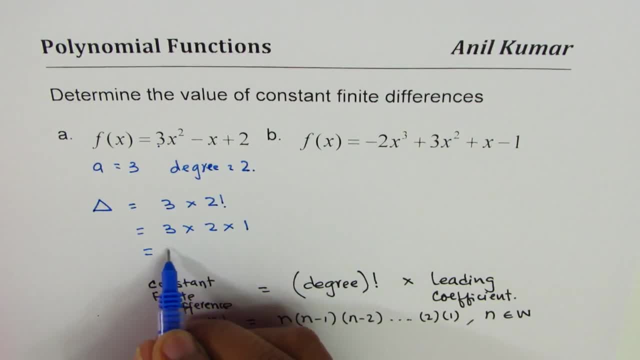 So that gives you 3 times 2, 6,, 6 times 1, 6, 6.. So the answer is 6.. You can now pause the video and answer the second one. You know how to do it right. Okay, that would be a good practice. 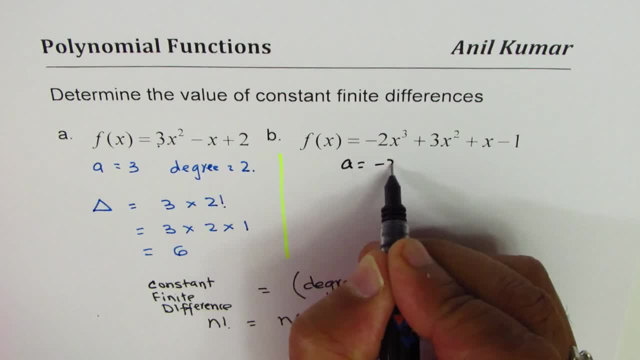 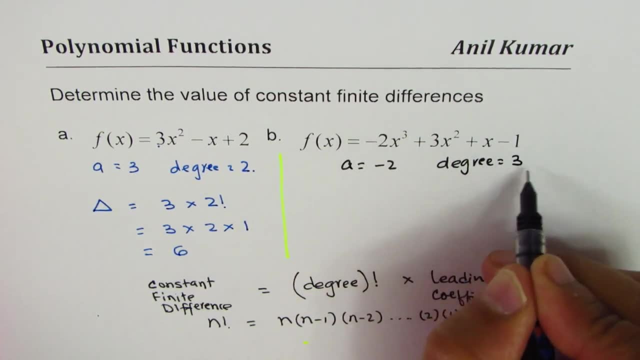 Now here, what is the value of a? The value of a is minus 2, leading coefficient right And the degree is 3.. Therefore, the constant difference, which is definitely the third constant right, This is second. Let me write here: 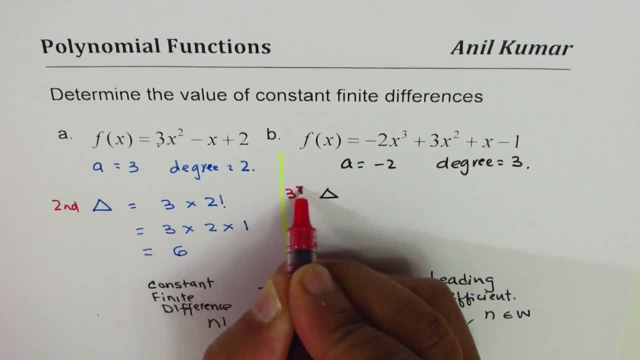 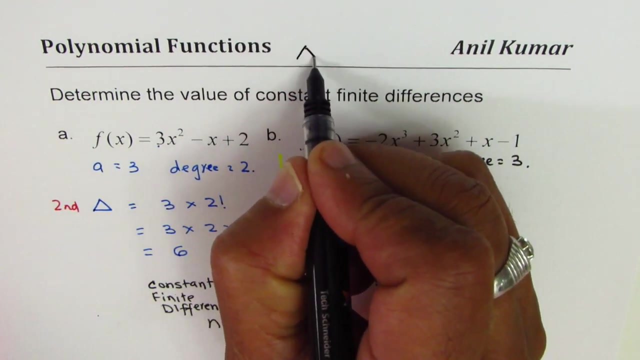 Second constant difference: right, This is the third constant difference Should be how much? It should be a times. we could also rearrange, right? So normally it's written a times n factorial where n is the degree. okay. So let me write down here: the constant difference is a times n factorial where n is the degree okay. 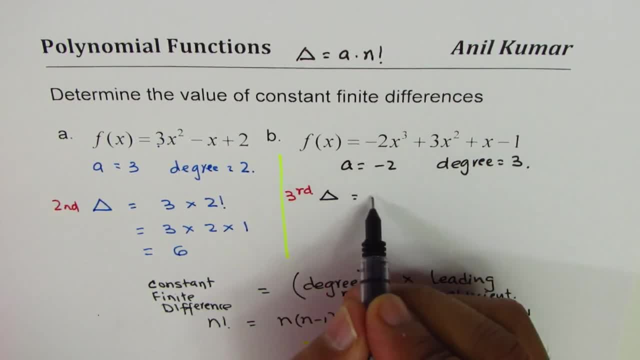 Let me write degree n, So a is minus 2 times 3 factorial times 3 factorial, is it okay? Okay, Minus 2 times 3 times 2 times 1, and that gives you 4 and 3, 12.. 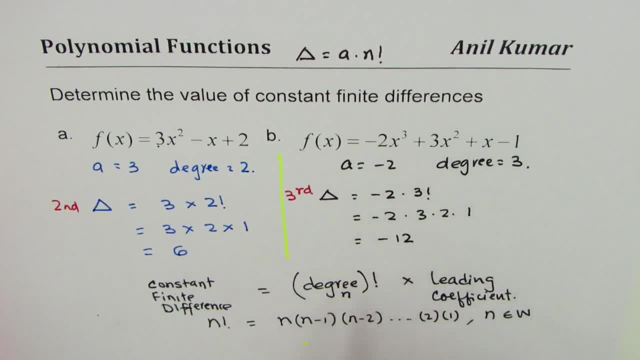 So minus 12, is your answer right? So the constant finite difference for the second one is minus 12, for the first one it is 6.. So with the help of formula you can very easily calculate finite difference for any polynomial. 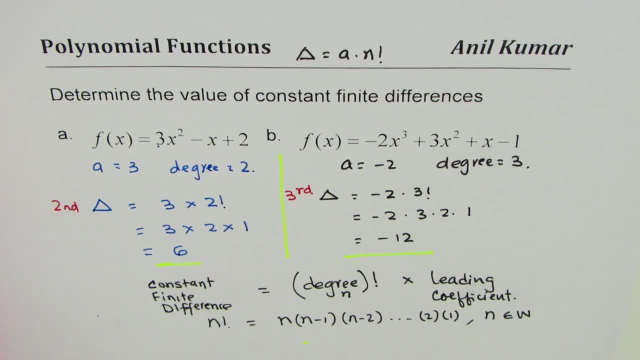 The constant finite difference for any polynomial right. So the constant finite difference is product of leading coefficient and factorial of its degree. n factorial right. I hope that helps. I'm Manil Kumar. You can always share and subscribe my videos. 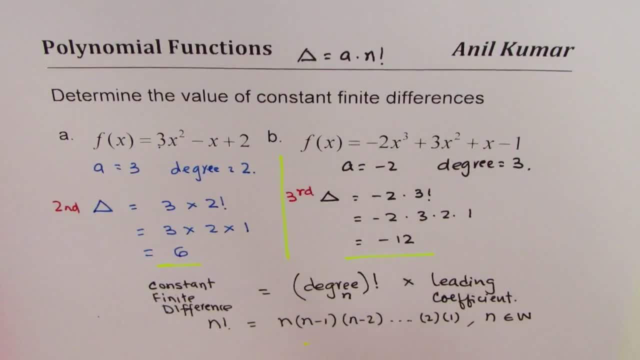 Feel free to post questions. Thank you And all the best.